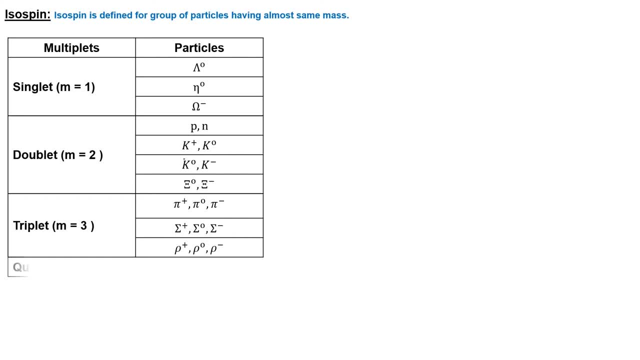 mesons particles are almost same, These are called triplet. The masses of all the four delta baryon particles are also same, These are called quadrant Isospin. defined for these groups, group are called multiplates and their multiplicity is given by 2i plus 1, where i is the isospin. 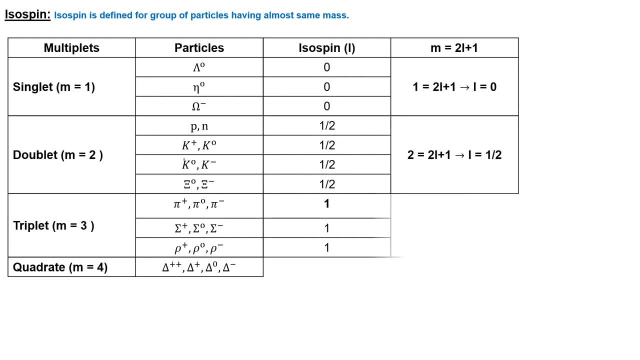 So isospin is 0 for singlet, half for doublet, 1 for triplet and 3 by 2 for quadrate. Another important thing is that here isospin is defined only for hadrons. This is because only hadrons interact with strong force, not the leptons. 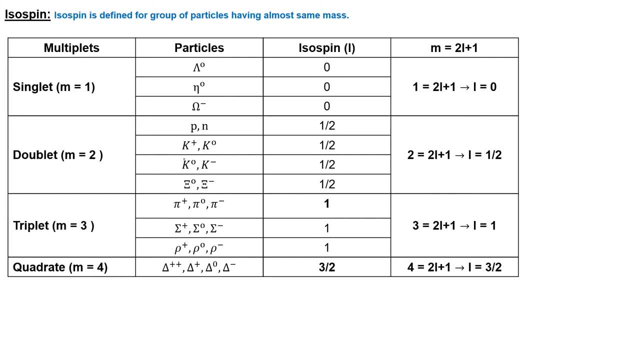 Talk about leptons. isospin has two different generations: strong and weak generation. Here all the particles of which we have defined isospin. this is their strong isospin. Strong isospin is not defined for leptons, But still if leptons are participating in nuclear reaction, their strong isospin considered. 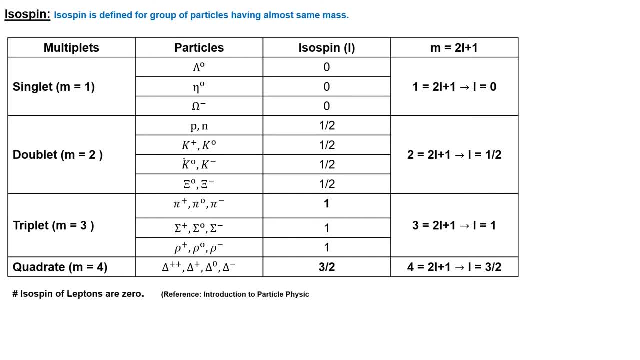 to be 0. But weak isospin is defined for leptons. But here we do not go into such detail And restrict ourselves to strong isospin. Like the leptons, all gas boson particles such as photon, W and G boson also have strong. 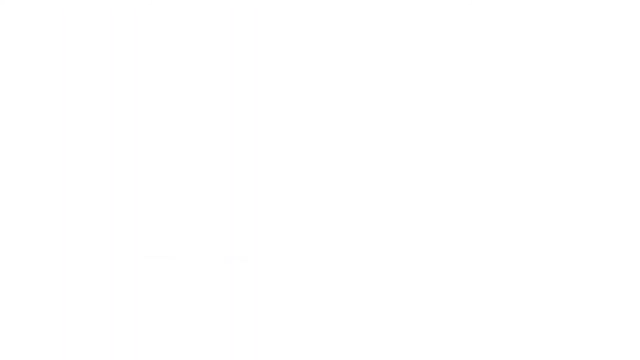 isospin 0.. In isospin, spin does not mean the spinning motion of the particle. Rather, this quantum number has given this name only because, like the spin, isospin also has values integer or half integer. Isospin is the dimension of angular momentum, while isospin is a dimensionless quantity. 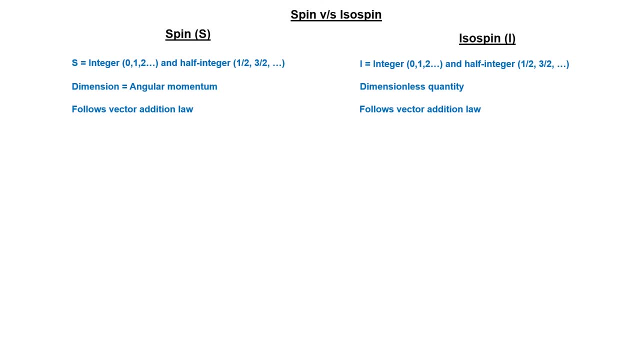 Like this spin, isospin also follows vector addition law. According to isospin conservation, a total isospin must remain conserved in a nuclear reaction Like two protons decaying to kion and sigma. Both protons and the kion are the members of the doublet group, having isospin half. 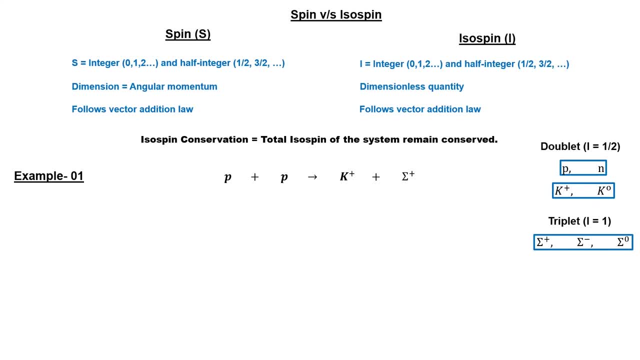 while the sigma is a member of a triplet group, So the isospin must be conserved in a nuclear reaction, like two protons decaying to kion and sigma. The possible total isospin of the both parent particles can be 0 or 1, while the possible 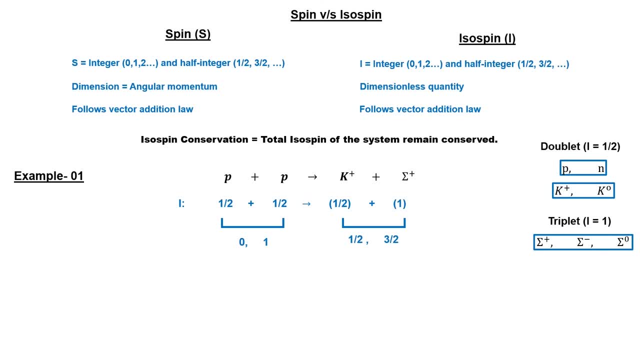 total isospin of the both daughter particles can be 1 by 2 or 3 by 2.. Since no total isospin of parent particles matches with the daughter particles, That means isospin is not conserved in this decay reaction. 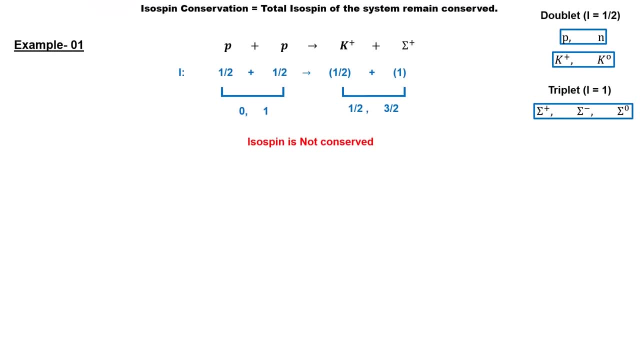 In the next example, the decay of two protons is taking place in a nuclear reaction like kion and sigma. protons is taking place in proton, sigma and kion. Again, since proton and kion are the members of the doublet group, they have isospin half, while the sigma is a member of the triplet. 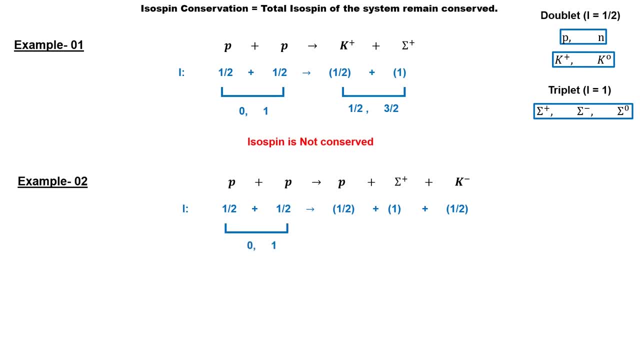 group, so its isospin will be 1.. The possible total isospin of both parent particles is 0 or 1.. While talking about the daughter particles, possible total isospin of the proton and sigma may be 1x2 or 3x2.. In this, if we do vector addition of the isospin of kion, then the 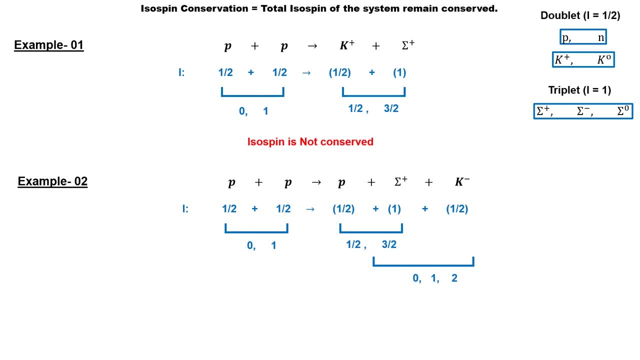 total isospin of the daughter particles may be 0,, 1, or 2.. Since the total isospin of the parent particle is matches with the total isospin of the daughter particles, so the isospin is conserved in this reaction. Again, comparing spin and isospin: isospin: 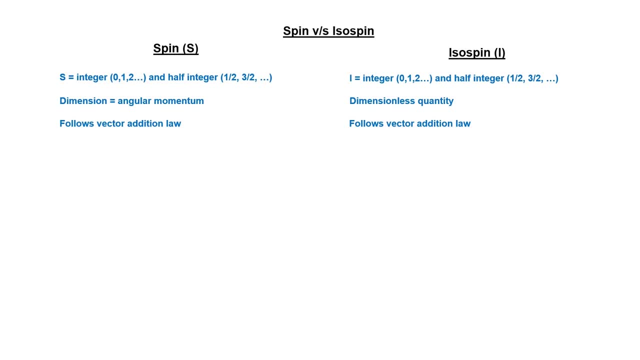 also has projection like this spin, but in spin projection is denoted by g component of the spin, while in isospin it is called the third component of isospin. For members of any multiplet group having isospin i, the values of the third component of isospin may vary from plus i to minus i, For example the proton and neutron doublet group have isospin half. but the proton has a third component of isospin plus half, while for neutron the third component of isospin is minus half. Similarly the isospin of pion triplet group is one. so the third component of isospin of pion plus has plus one pion zero has. 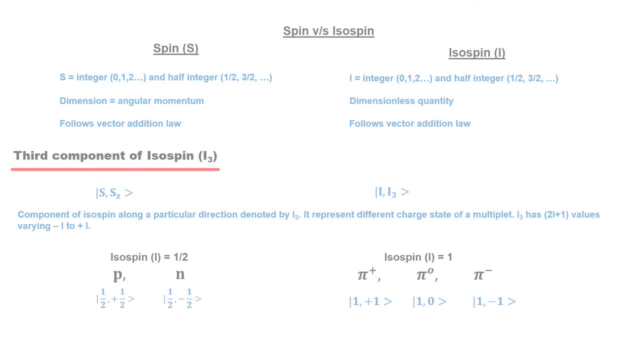 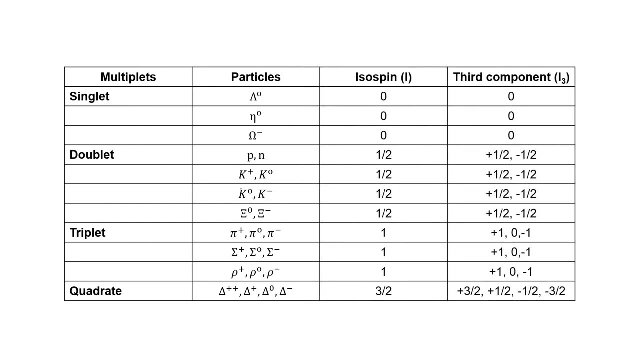 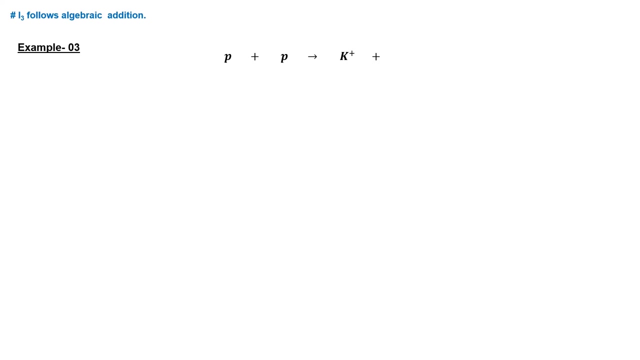 zero, while pion minus has minus one. Here, for all hadron particles, the third component of isospin is defined. The third component of isospin follows the algebraic addition rule, Such as the interaction of two protons indicate two kion and sigma baryon. In this decay both. 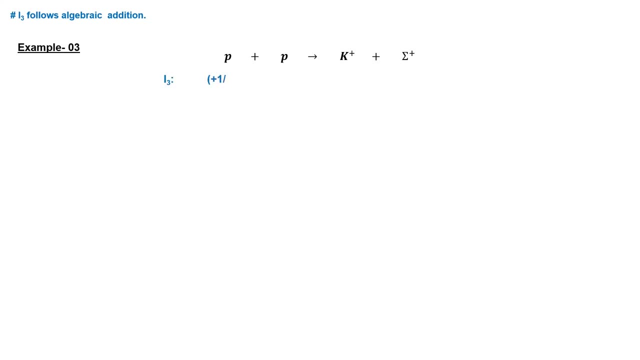 proton and kion are the particles of doublet group having third component of isospin plus half, whereas sigma is the particle of a triplet group having third component of isospin plus one, Since the total i3 of the parent particle is not equal to the total i3 of the daughter particles. 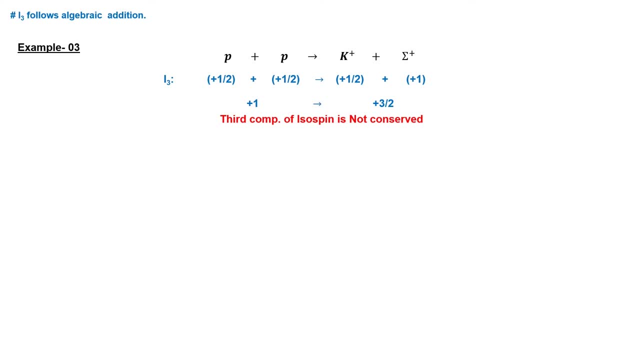 that means the third component of i is not conserved in this reaction. In the next example the interactions of proton and neutron are decaying into lambda and sigma particle. The proton and neutron have i3 plus half and minus half respectively, while lambda zero is a singlet. 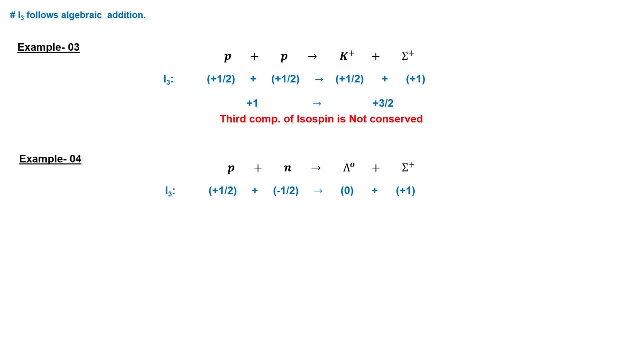 particle having i3 is zero and sigma plus have i3 plus one Again. in this reaction the third component of isospin is not conserved. As we learned, the proton and neutron have isospin half. But how can one calculate the isospin of a nucleus, a system made from a combination? 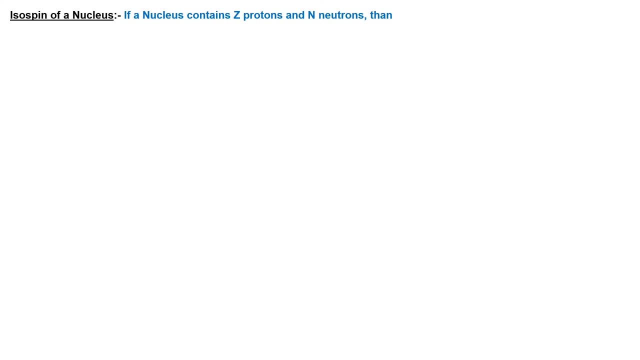 of proton and neutron. If a nucleus had g protons and n neutrons, the third component of the isospin of that nucleus is given by g-n, by 2. And the maximum isospin of the nucleus is the half of the mass number. 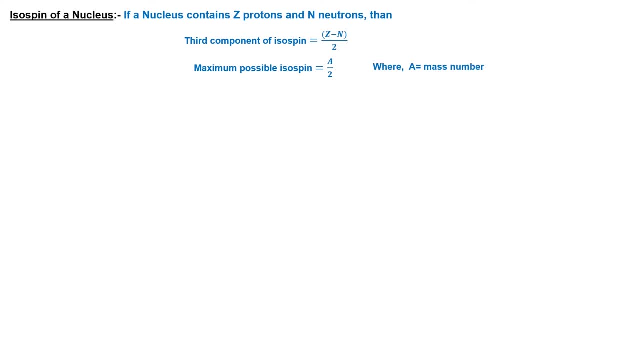 Such as nucleus of the helium, Such as nucleus of helium. The helium nucleus consists of two protons and two neutrons, So the third component of its isospin will be 0 and the maximum isospin will be 2.. All isobars of any nucleus have the same isospin. 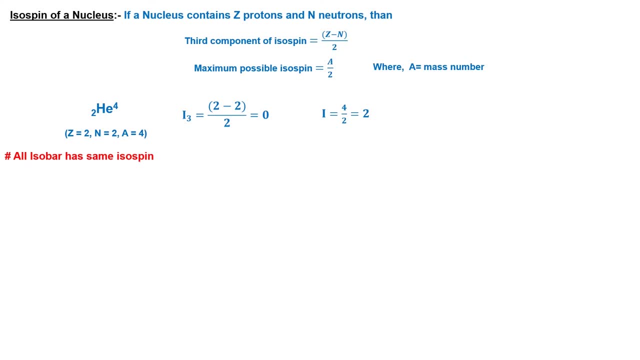 Isobars are such nuclei, those have same mass number, Such as carbon-14, nitrogen-14, oxygen-14.. These are the isobars of each other And their isospin will be 7.. But the third component of their isospin will be 7.. 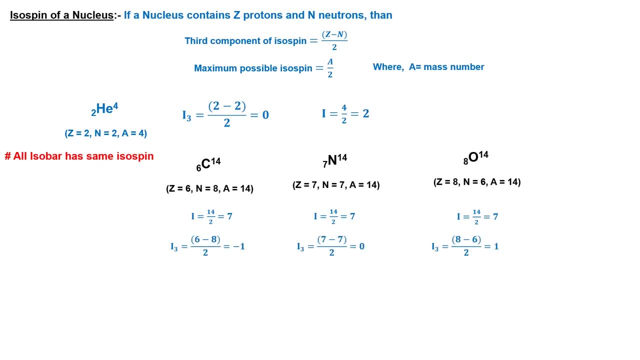 And their isospin will be different. But deuteron's isospin is slightly different from this concept. The deuteron is called the nucleus of one proton and one neutron. That means its maximum isospin should be 1.. But deuteron has isospin 0. 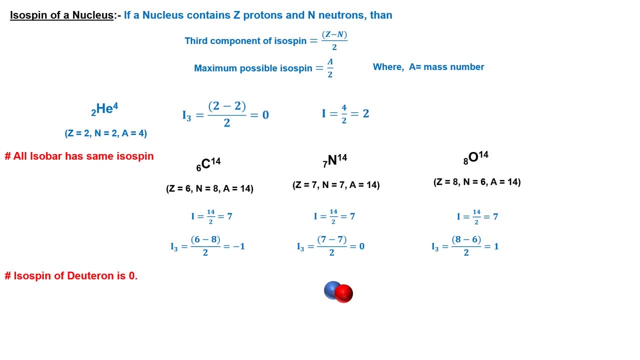 This is because if a particle has isospin 1, that means that particle is a member of a triplet group, But in deuteron one proton and one neutron together form two nucleons singlet system. That's why its isospin is considered zero.